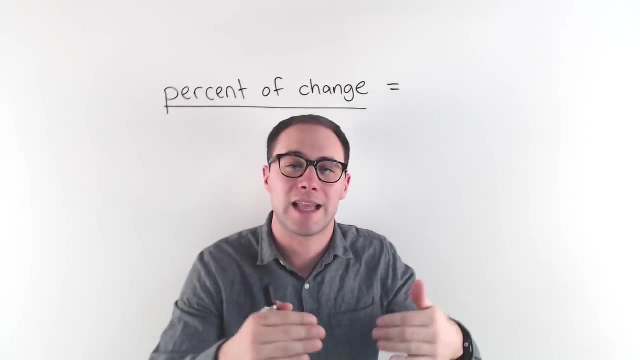 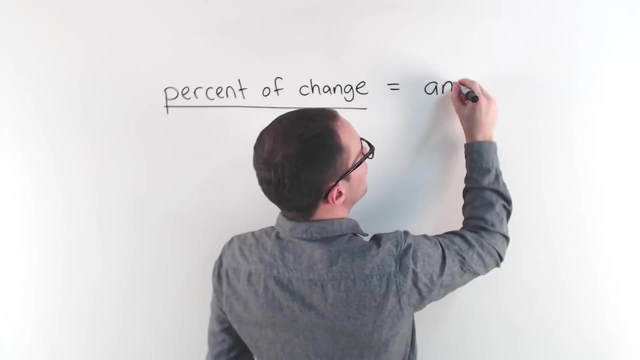 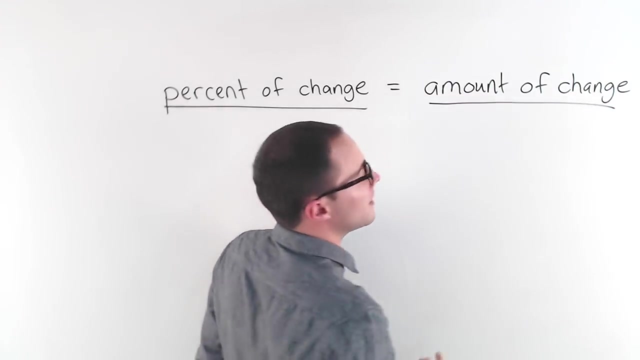 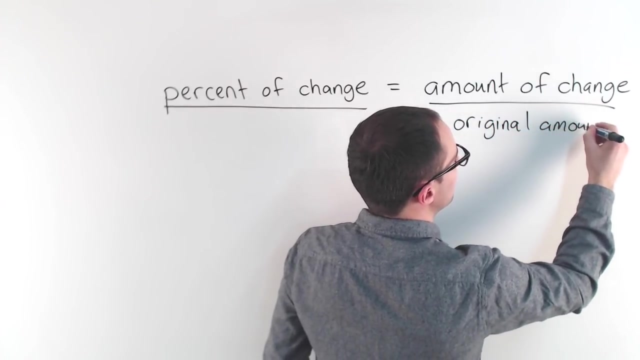 Sometimes it will be a percent of decrease if the amount is less than the original. So percent of change is pretty simple. All you do is look at the amount of change, So the new amount is divided by the original amount, And again, just use some logic. 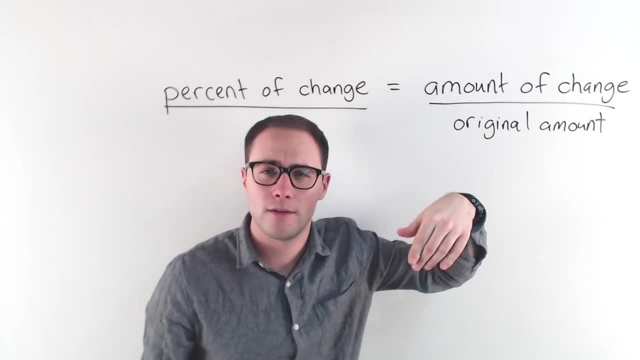 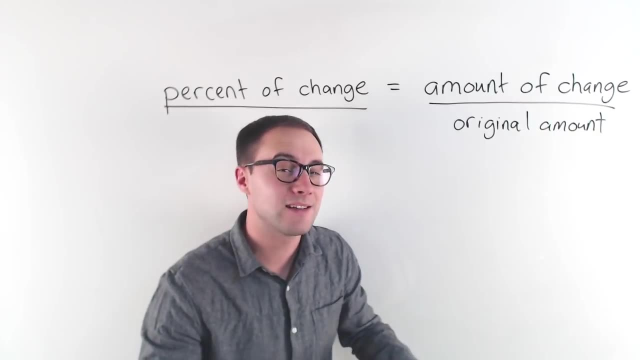 If the new amount is more than the original amount, well then, you've got an increase, a percent increase. If the new amount is less than the original amount, well then, a decrease. right, You have a percent decrease. Let's try our first example. 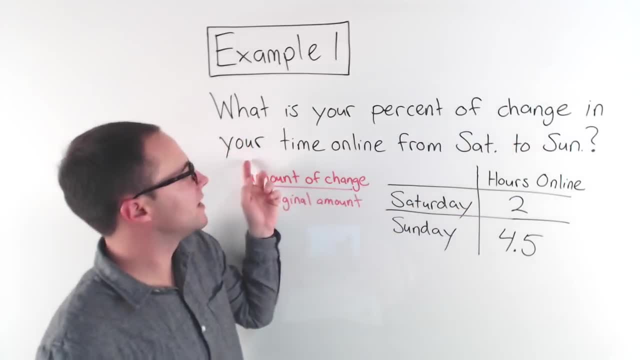 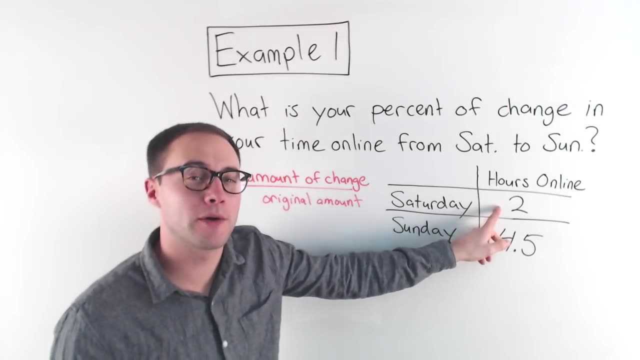 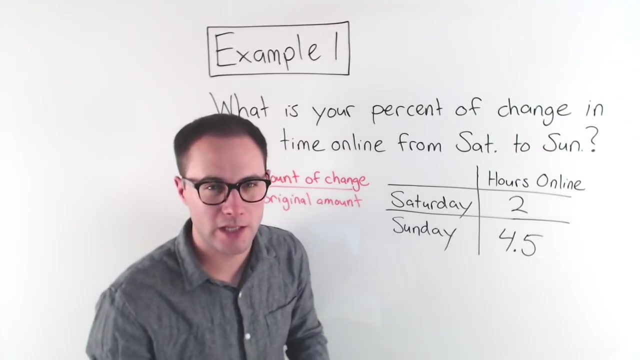 Here's example 1.. What is your percent of change in your time online from Saturday to Sunday? So here's a little table. On Saturday, we spent two hours online surfing the net. On Sunday, four and a half hours online. So what is that percent of change? 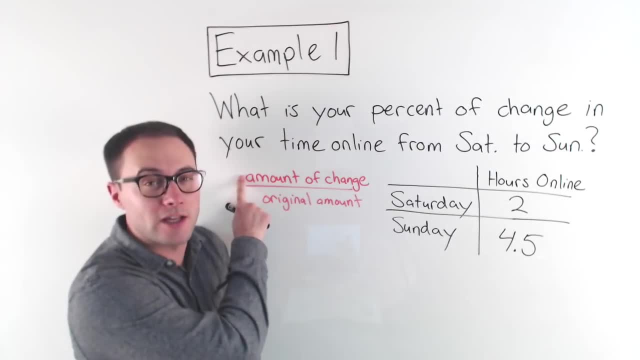 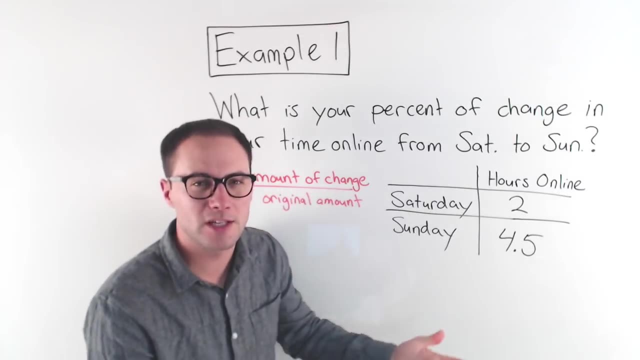 Well, if we remember, percent of change is the amount of change over original amount, And then we're going to make that into a percent. So what's the amount of change? How much did it change? Well, we started. We're going from Saturday to Sunday. 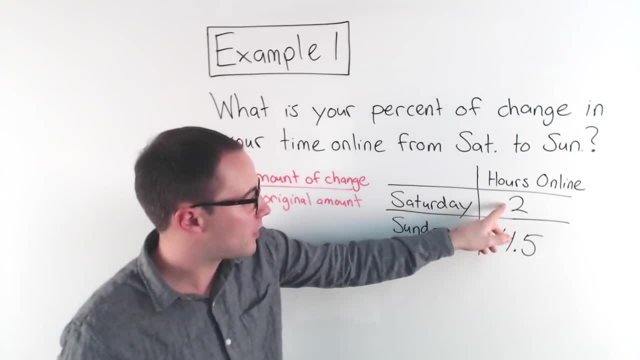 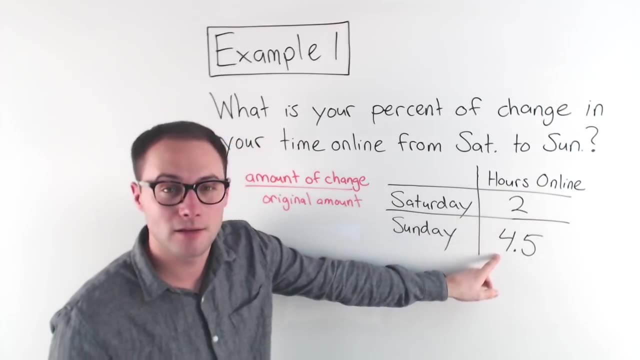 Saturday was two hours, Sunday was four and a half. So how much did it change? Well, it increased. So we know this is going to be a percent increase. It increased by two and a half hours, So that 2.5 goes in my numerator. 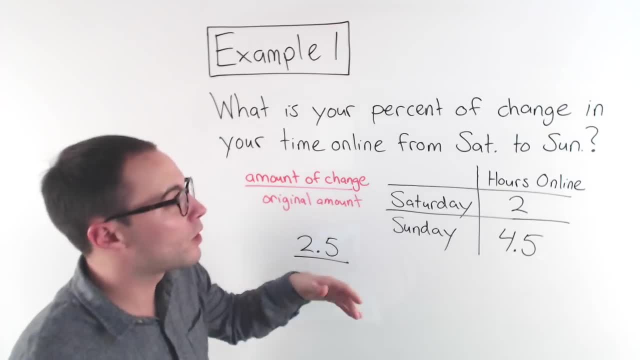 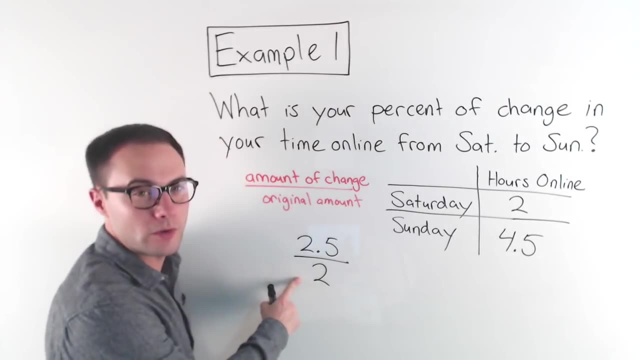 In the denominator what's my original amount. Well, where did I start? I'm starting from Saturday. That's my original, So I'm going 2.5 over 2.. Okay, Now this doesn't look like a percent, right. 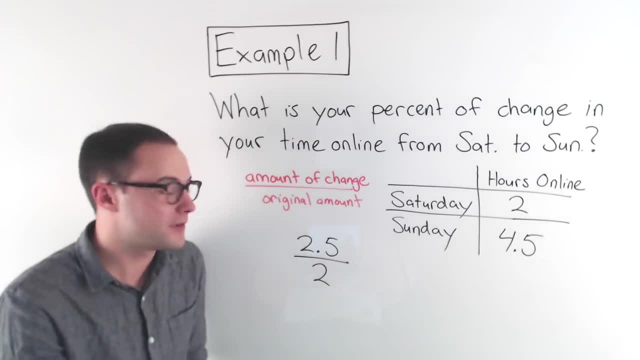 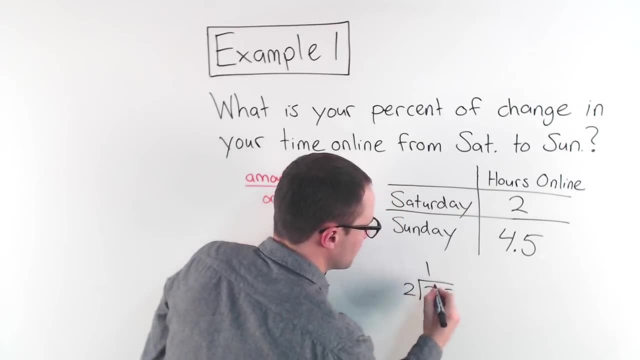 So let's get to a percent. So first I'm going to do that division, I'm going to do 2.5 divided by 2.. 2.5 divided by 2.. Well, that goes in: one Get zero. 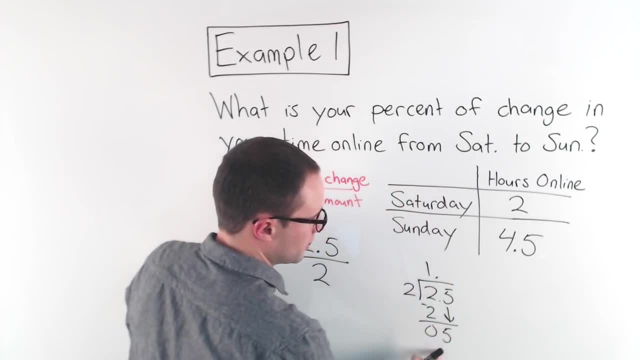 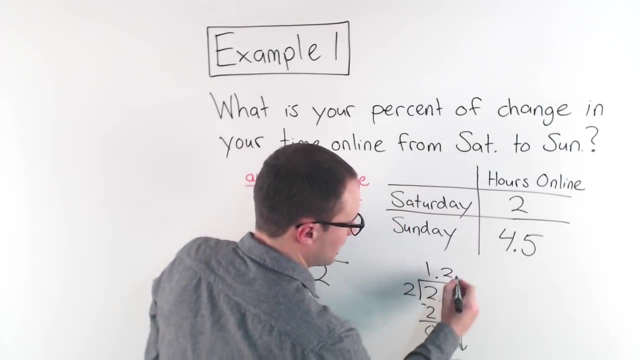 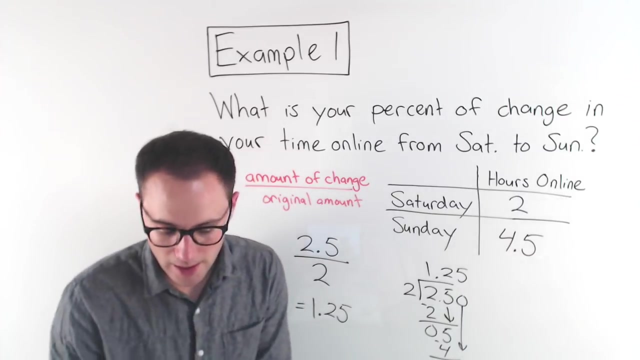 Bring down the five. There's my decimal. Two into five is two, That's four. Subtract I get one. Add a zero. Bring it down. Two into ten is five, So I get 1.25.. Again, that does not look like a percent either. 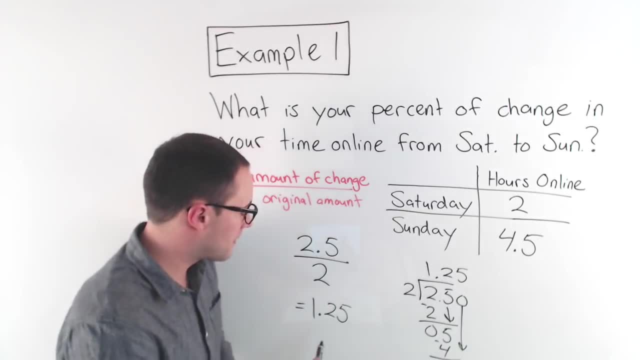 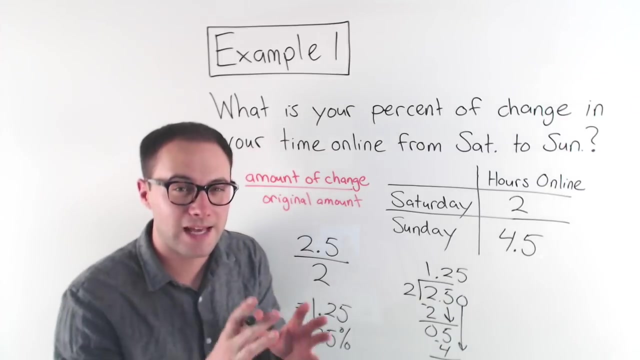 How do we change decimals to percents? Hopefully you remember. Well, we just moved the decimal point twice to the right, which means that becomes 125%. Now I'm not quite done, because 125% that's half of it. I got to remember. 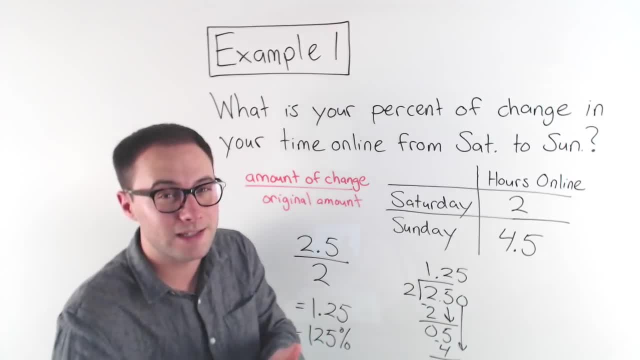 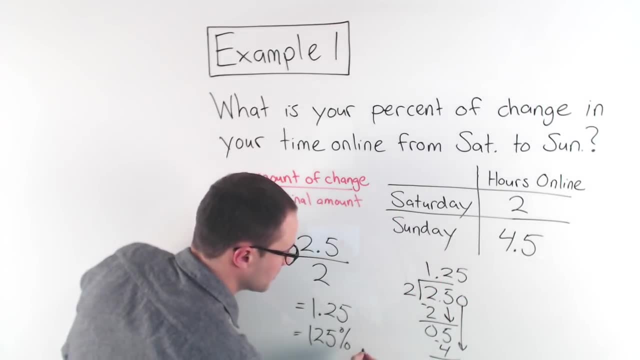 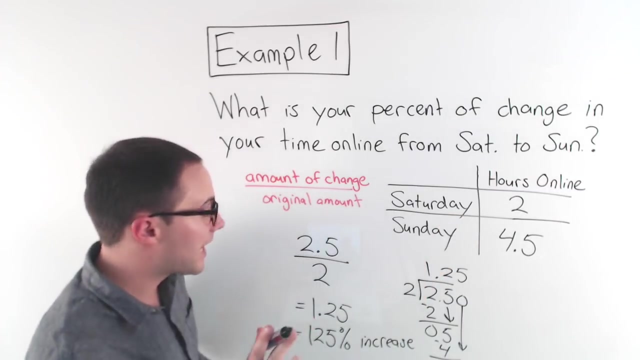 Is 125% increase or 125% decrease in change. Well, we remember that from Saturday to Sunday we increased, So that is 125% increase. Increase of hours online. Now you might also be looking at this and think. 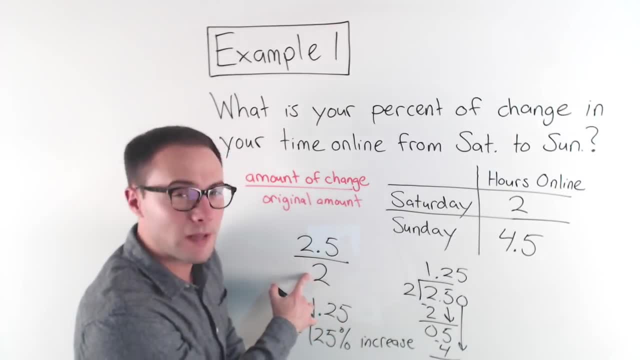 well, did I have to divide it like that, Couldn't? I have just maybe made this over 100?? And yeah, you could If you notice that, great. So remember, if we have a fraction, if we can somehow get the denominator to 100,. 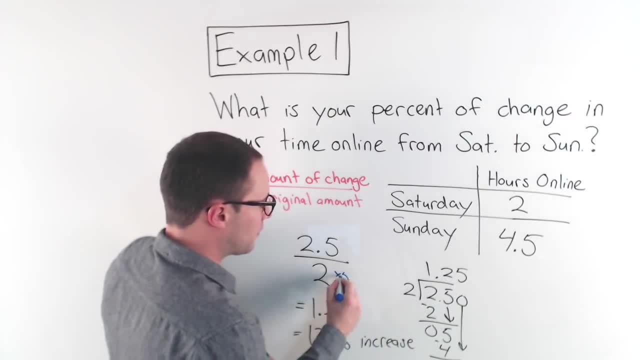 then it's really easy to change to a percent. So if I multiply the numerator and denominator by 50, I could also that becomes 100.. 2.5 times 50, well, 2 times 50 is 100. 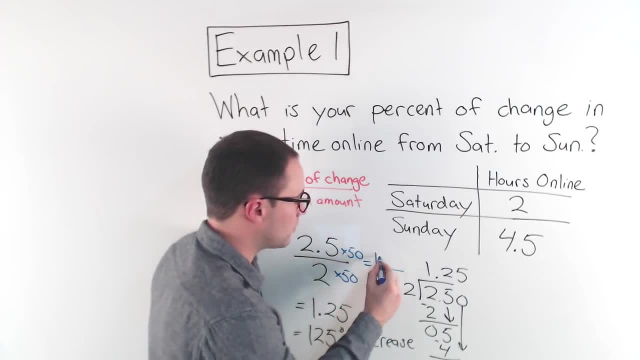 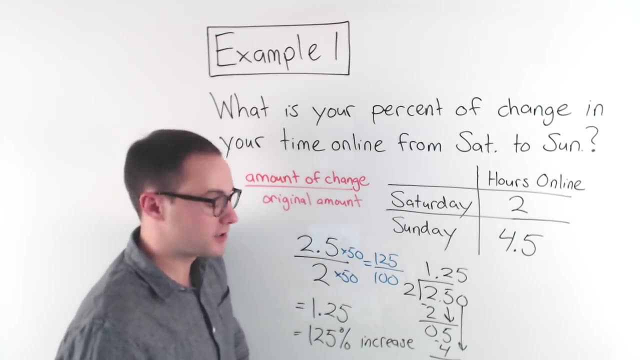 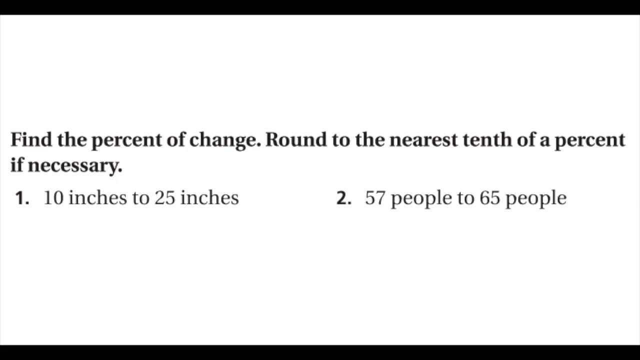 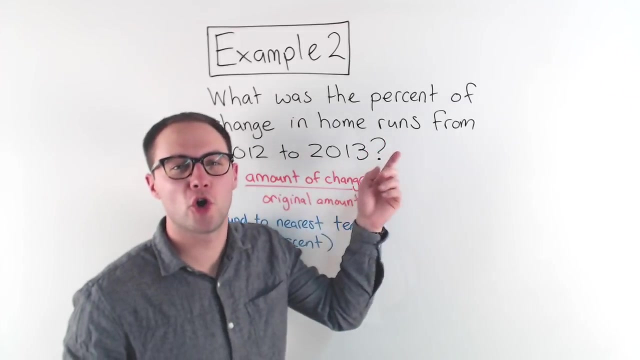 Half 0.5 times 50 is 25,, so that's 125.. 125 over 100,, 125 per 100. 125 percent. Here's something to try on your own, All right. example two: What was the percent of change in home runs from 2012 to 2013?? 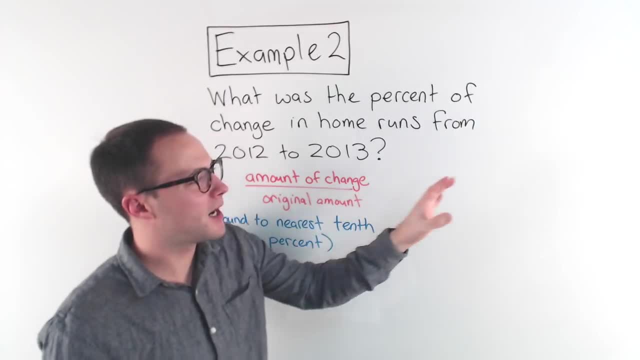 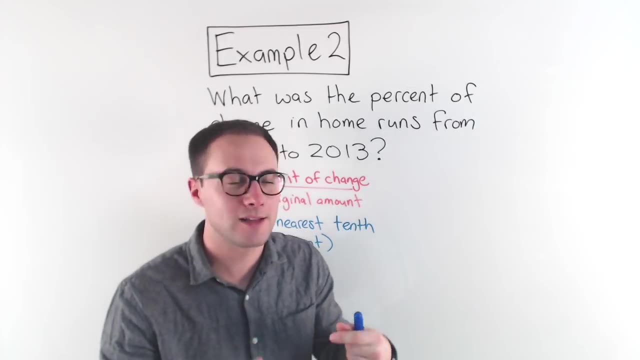 So let's look at the table over here. You can notice: in 2012, there were 28 home runs. In 2013, there were only 20.. So right off the bat you should realize that this is going to be a percent decrease. 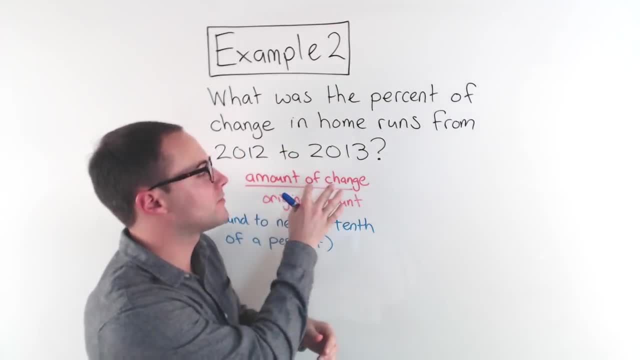 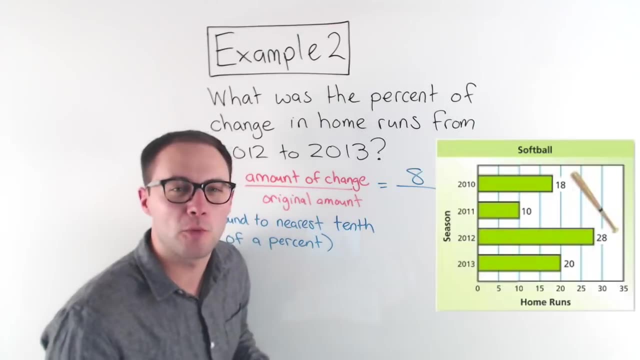 Well, how much did it decrease? by What was the amount of change? From 28 home runs to 20?? Well, that change was 8.. It decreased by 8 home runs. What was the original amount? Well, we're starting in 2012.. 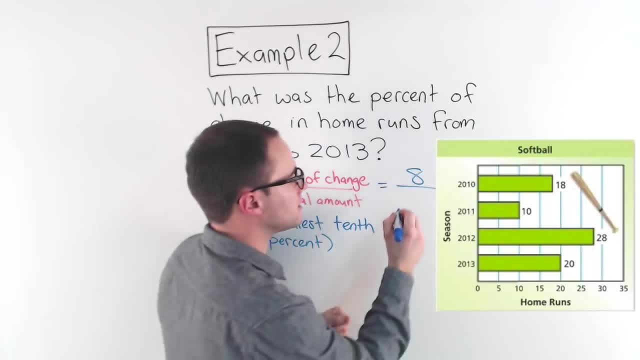 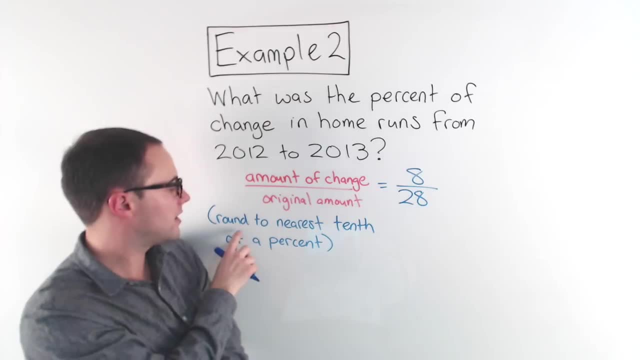 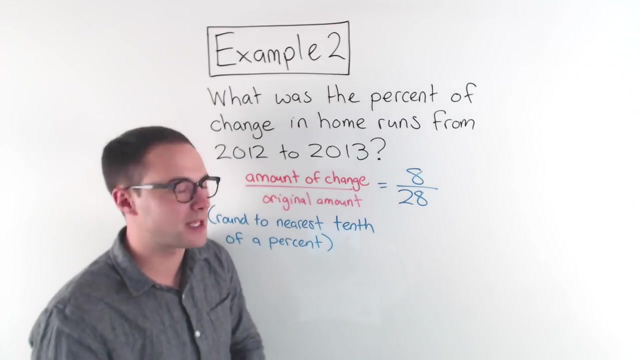 So in 2012, there were 28 home runs, So 8 over 28.. Now we just need to convert that to a percent And if you notice, here it says round to the nearest tenth of a percent. In case we get decimals that keep going, we can round to the nearest tenth of a percent. 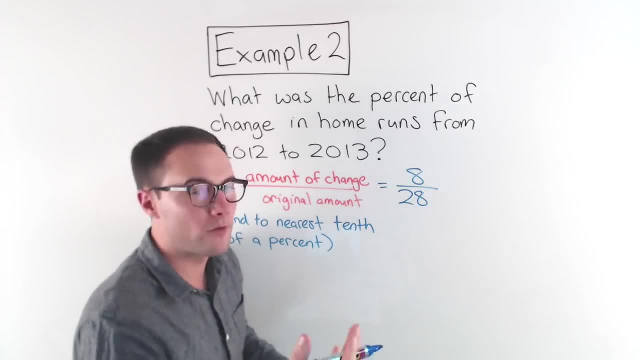 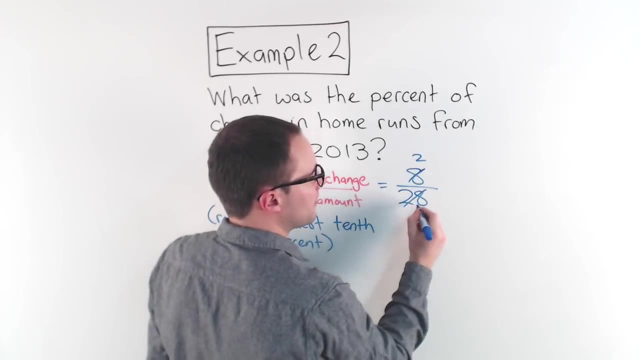 Now to make my life a little bit easier, I'm going to simplify this before I start to do my long. division 4 is a common factor of 8 and 28.. So that would become 2, and that becomes 7.. 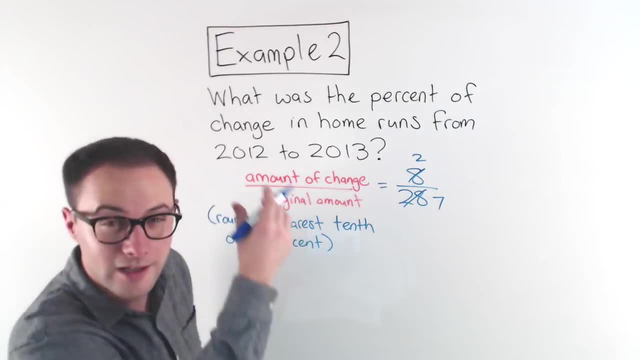 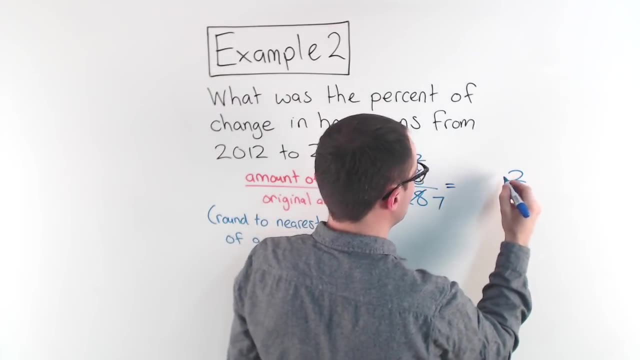 So now I've got to convert 2 sevenths into a percent, And to do that, the first step is to change it to a decimal. So I'm going to do some long division. I'm going to get 2 divided by 7.. 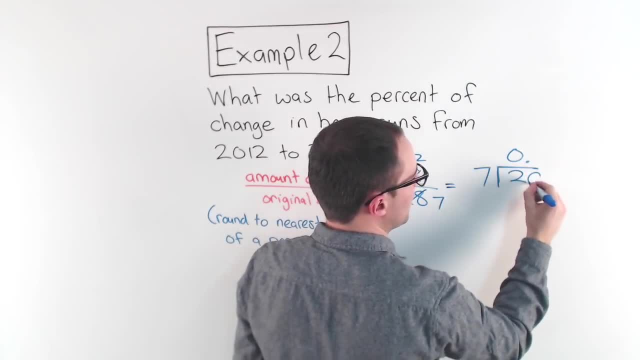 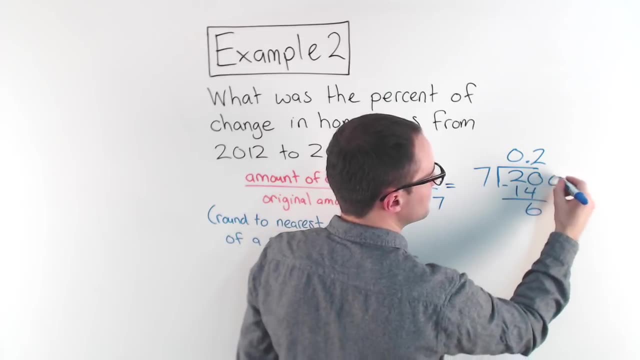 Well, 7 into 2 goes 0 times. So I'm going to add my decimal at a 0.. 7 into 20 goes twice, That's 14.. Subtract, I get 6 at a 0.. 7 into 60 goes 8 times. 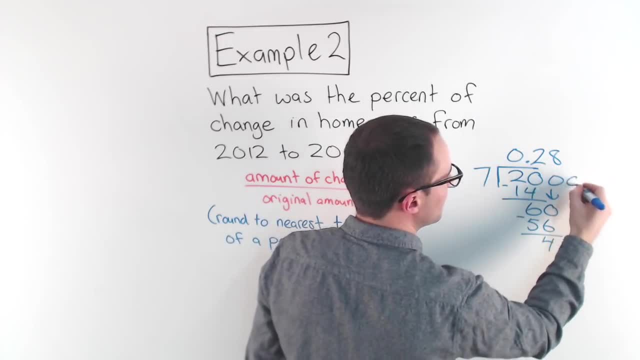 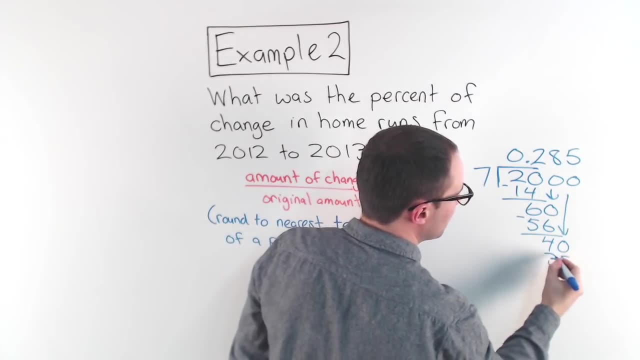 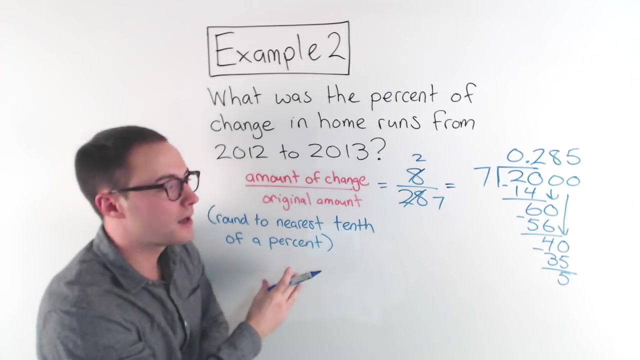 That's 56.. Subtract, I get 4 at another 0.. 7 into 40,, 5 times That's 35.. Subtract, I get 5.. Now, remember You can round to the nearest tenth of a percent. 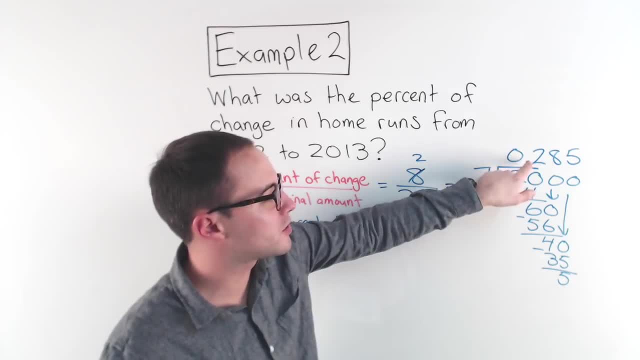 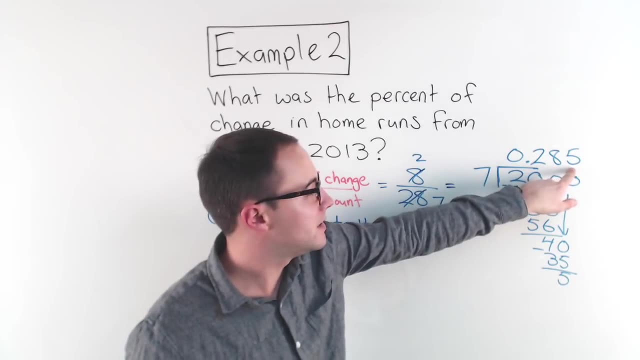 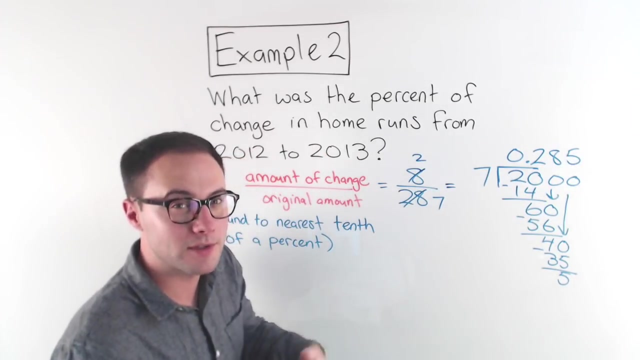 When I change this decimal to a percent, I'm moving the decimal point twice to the right, So I'm not quite far enough, because I don't know if this 5 needs to stay a 5 or round up to a 6.. I need one more number here before I'm able to stop. 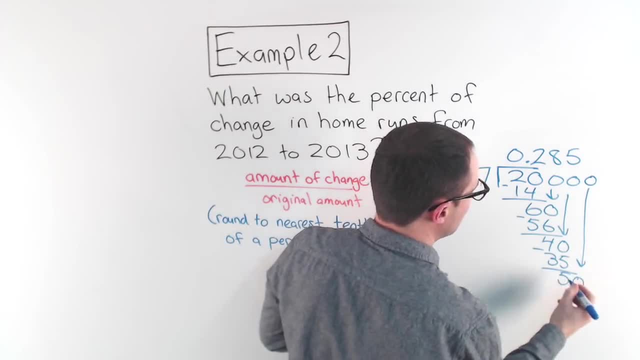 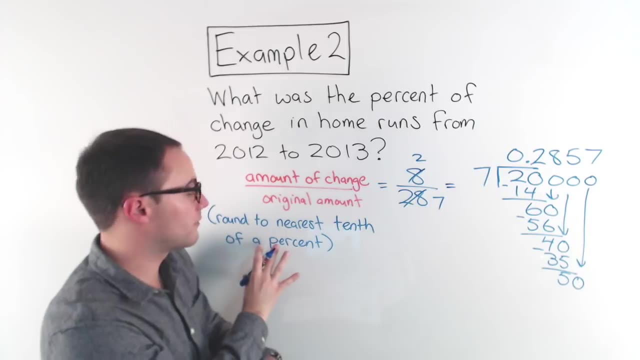 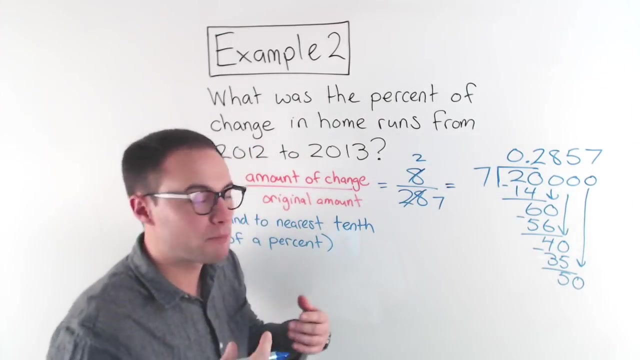 So add one more, 0. Bring it down 7 into 50.. 7 times That's 49. And I can stop there because I can round to the nearest tenth of a percent, So 0.2857 as a percent. 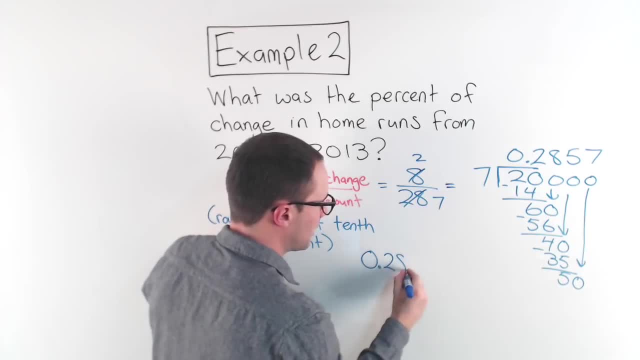 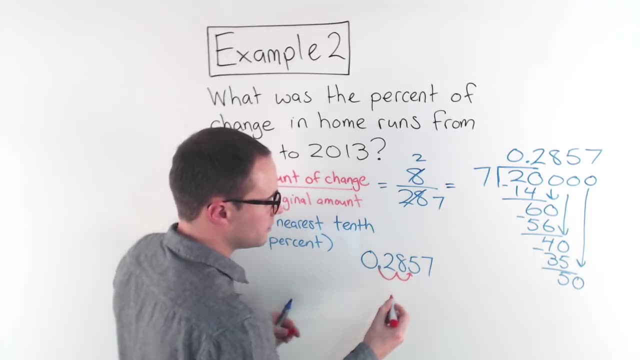 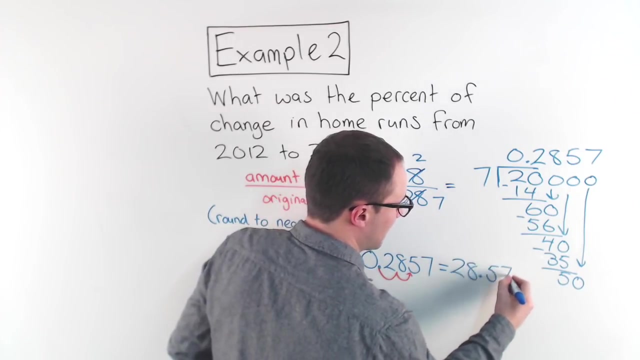 I'll just rewrite that 0.2857 as a percent. All I need to do is move the decimal point twice to the right, Which would give me 28.5.. 0.57%, But we want to round to the nearest tenth of a percent. 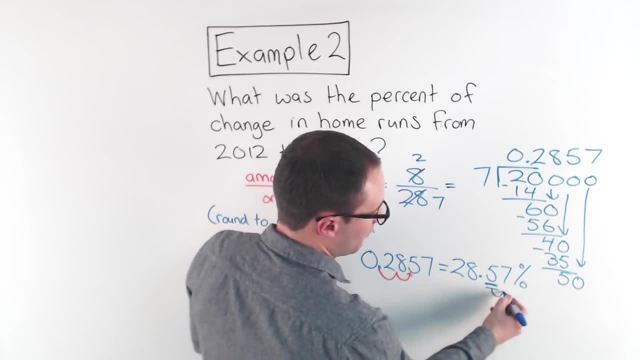 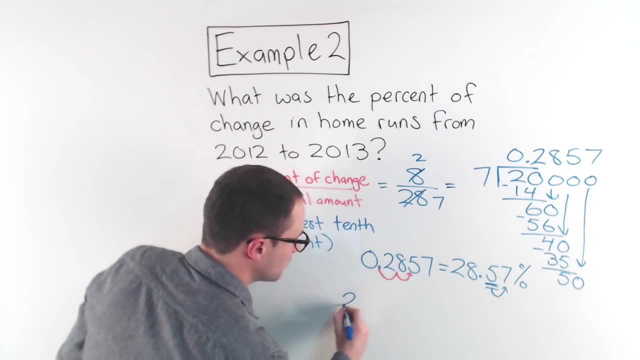 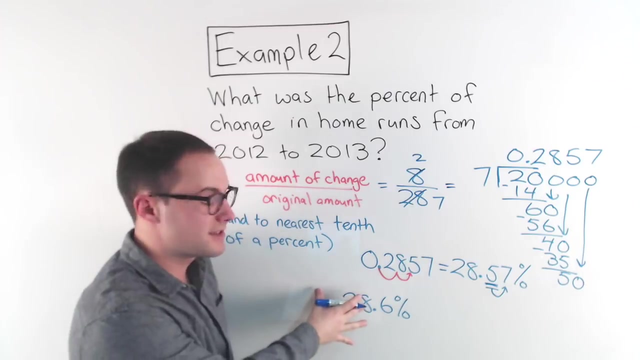 Which is right here. So am I rounding up, or is it staying at a 5?? Well, 7 is greater than 5.. So that becomes 28.6%. And last last step, Is this: a percent increase or decrease? 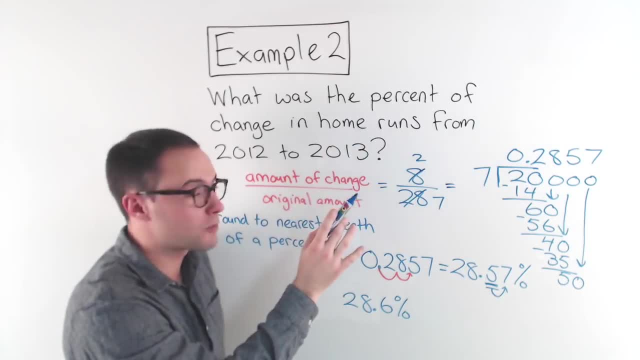 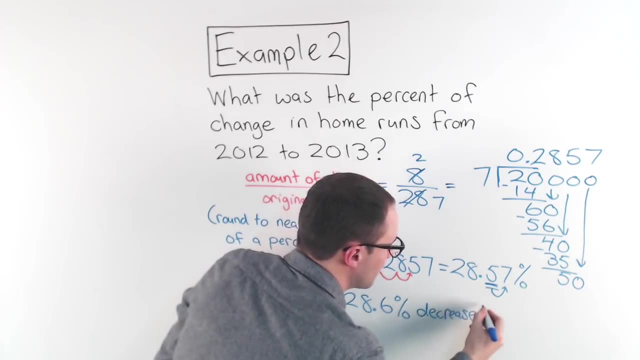 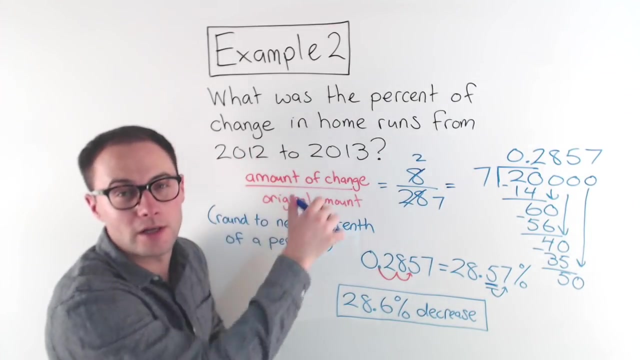 And remember, 2012 was 28 home runs, 2013 was 20.. It decreased. So that is my final answer: 28.6% decrease in home runs from 2012 to 2013.. Let's try one more example. 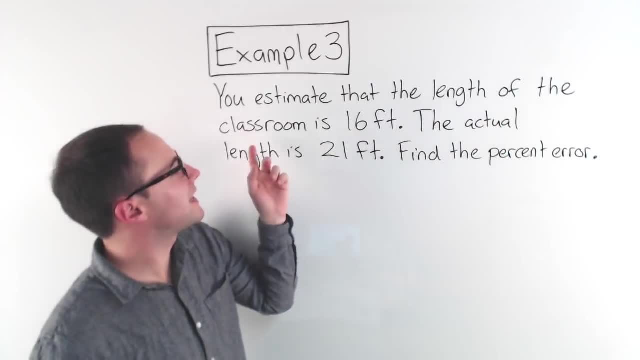 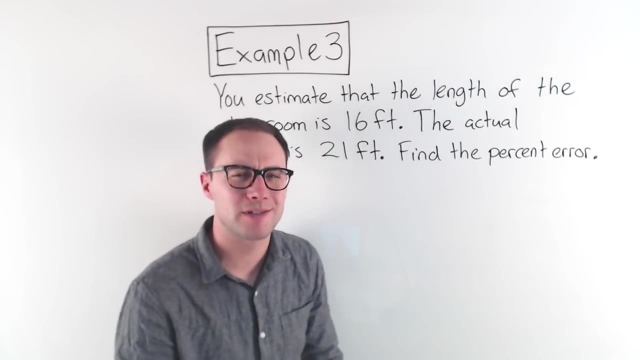 Here's our last example. You estimate that the length of the classroom is 16 feet. The actual length is 21 feet. Find the percent error. Well, we haven't talked about percent error, So let's first mention what that is. 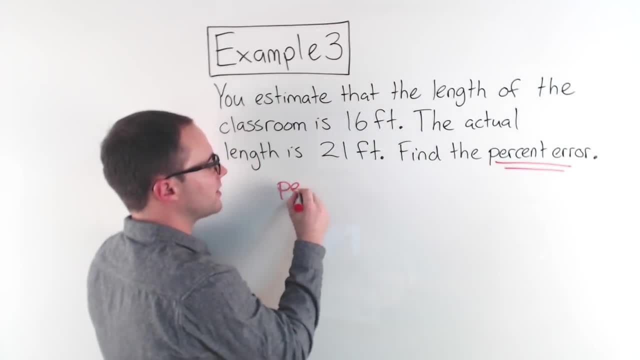 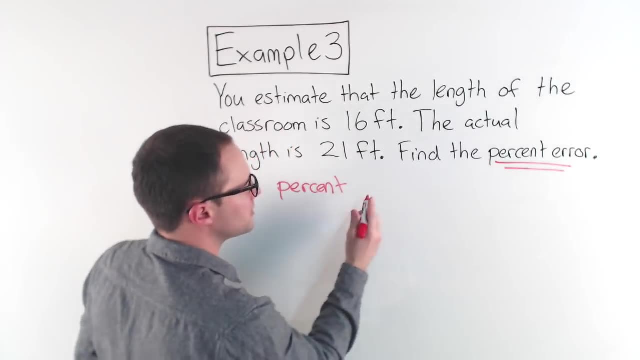 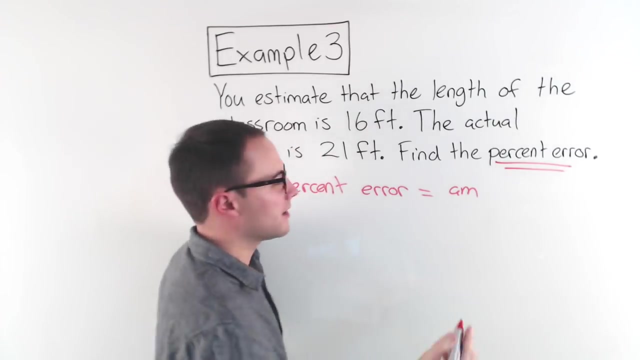 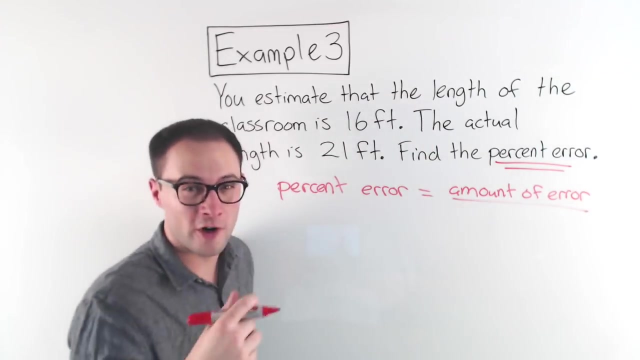 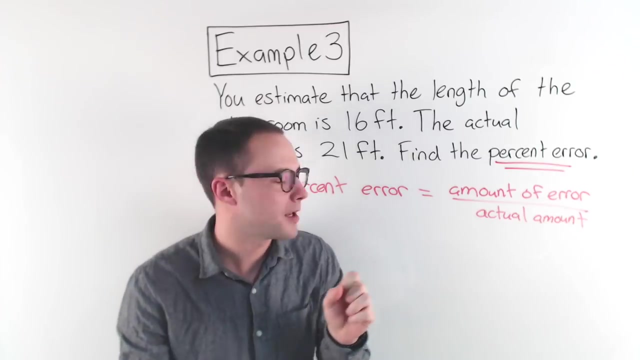 Percent error. Percent error is basically: what percent are you off by on your estimates? So percent error is just the amount of your error. How much are you off by Amount of error Over the actual amount? So the amount of the error? that's just saying, well, how much off is your estimate? 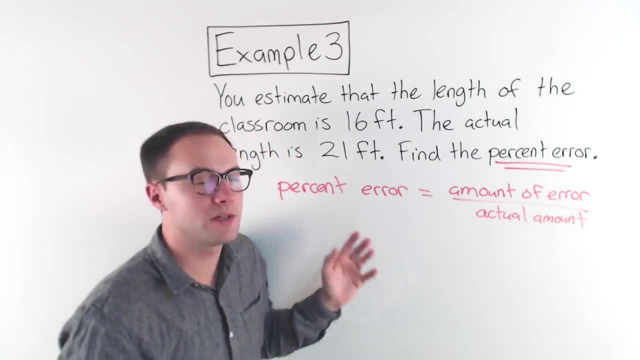 This is always going to be positive. You're never going to have a negative percent error. Sometimes your estimate might be too low, Sometimes it might be too high, It doesn't matter. That's always going to be a positive number. So, amount of the error over the actual amount. 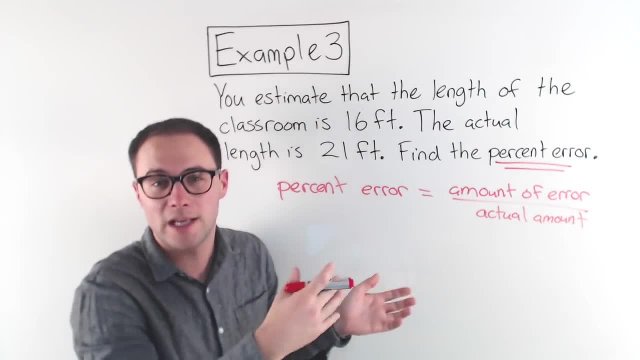 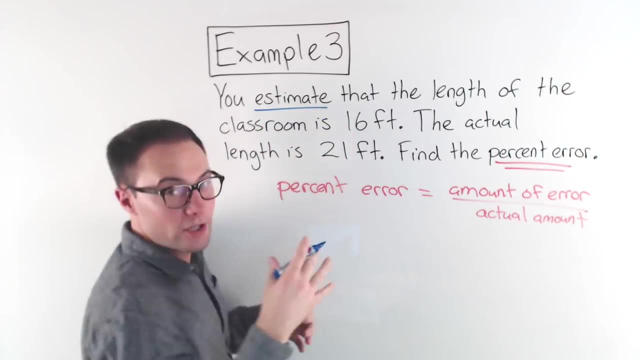 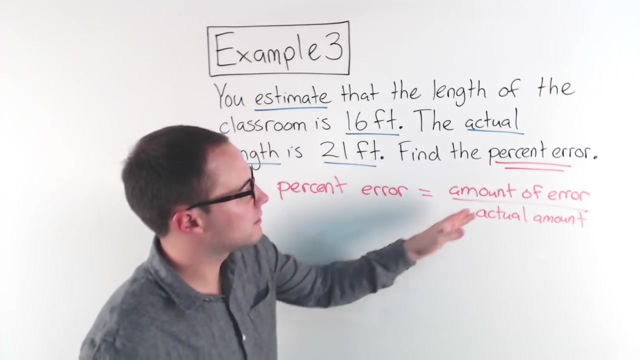 And then we write that as a percent, just like we do for percent increase or decrease. So let's figure this out: My estimate, or your estimate, was 16 feet. The actual length is 21.. Well, how much was our error? 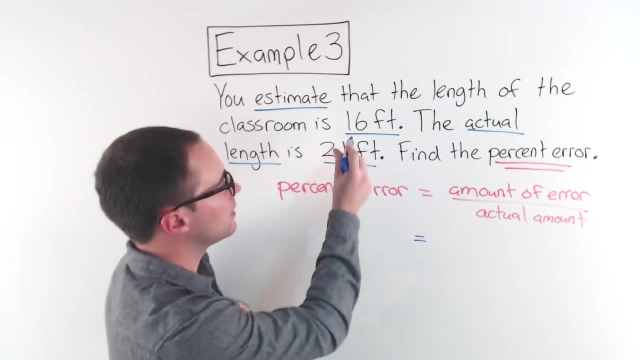 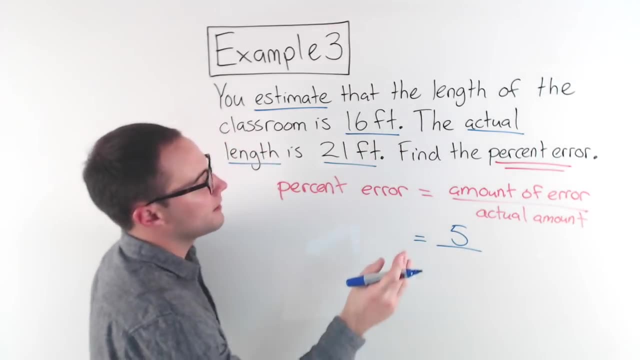 How far off were we? Well, from 16 to 21,. we were 5 feet off. That was our error. So 5 is our error. The actual amount, the actual length was 21.. So there's our fraction. 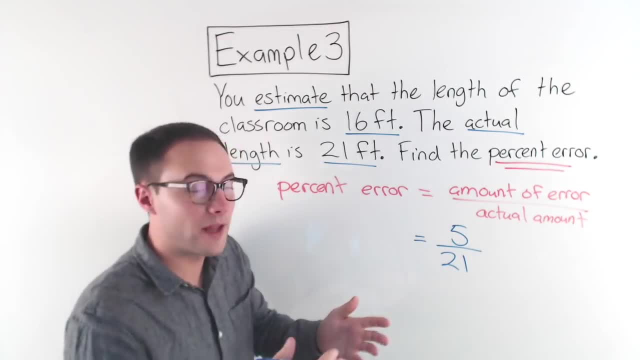 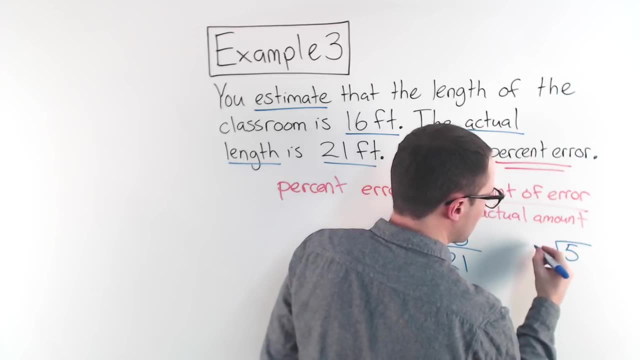 Now we just need to convert that into a decimal and then a percent from there. So let's do our long division. I'll just go ahead and do it over here: 5 divided by 21.. Well, that goes 0 times.